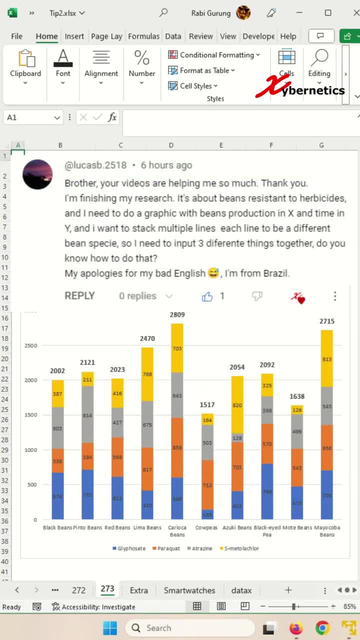 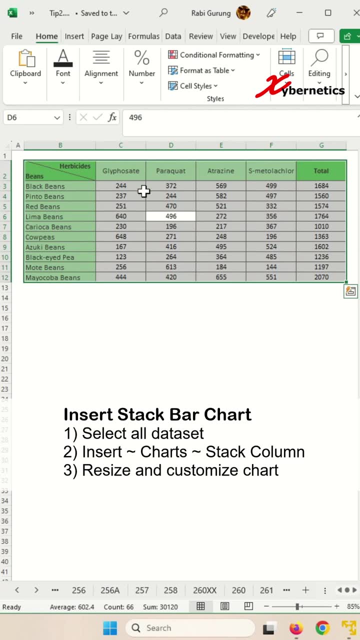 Recently one of my viewer inquired if I can demonstrate a stacked bar chart for his bean research program here. So this is how you do it. First you're going to place a cursor on your dataset table here. Press ctrl e to select the whole dataset, Click on insert charts and under 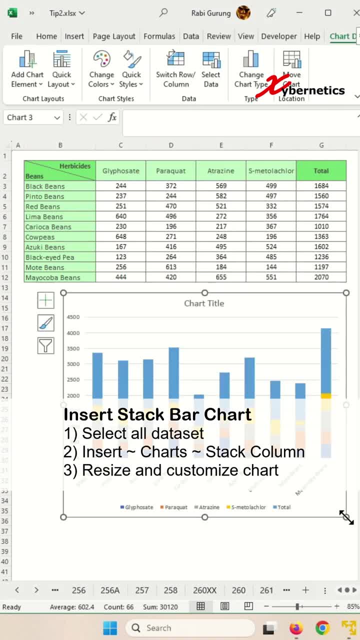 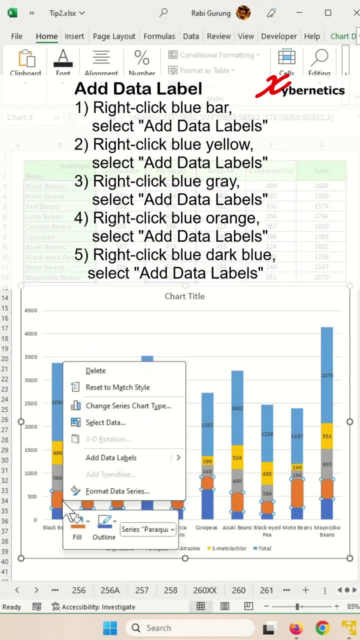 the bar charts. here, 2d column, you're going to select the stack and after that you're going to customize the bar chart a bit like this. After that, add some data label. Right click on the bar chart and add data label. Do the same thing for the rest of the bar charts. We know that the blue 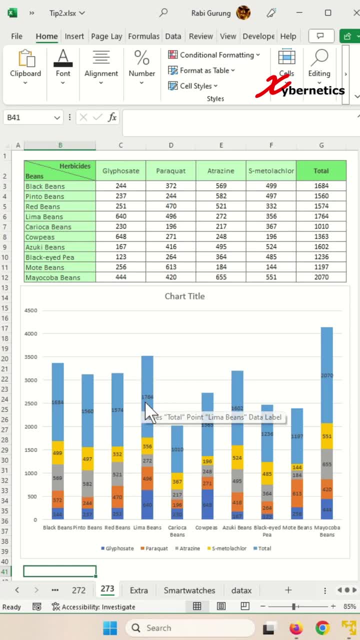 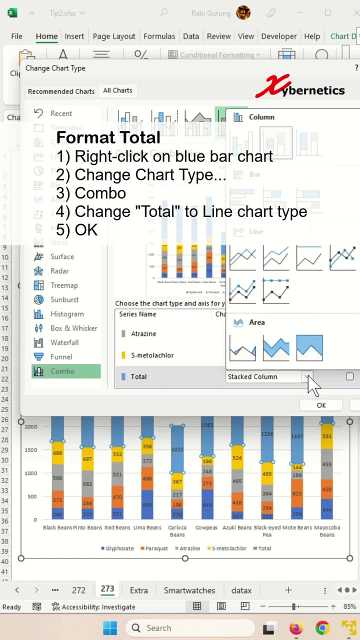 bar chart is your total itself. Let's make that into a data label only. So right click on the bar chart. Change the chart type. On this menu here you're going to click on combo. Scroll all the way down total. You're going to change this to a line and click okay, Now you're going to right. 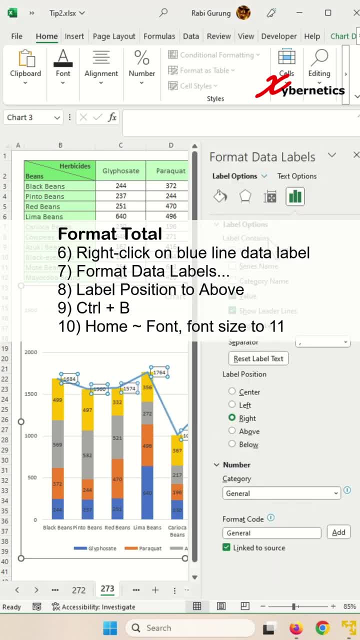 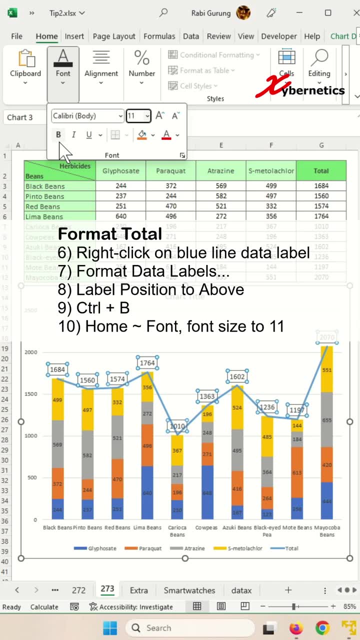 click data label for the total and you go data label like this, and over here you're going to say above, so that the numbers are right at the top here and basically go font. I'm going to change this font size to say 11 and make it bold, so it's obvious to read. Now to get rid of this line chart. 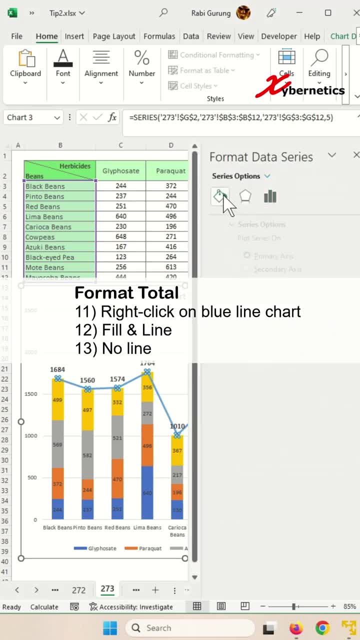 here: right click on your line chart here, Go data series again and go line and fill No line and you are done. 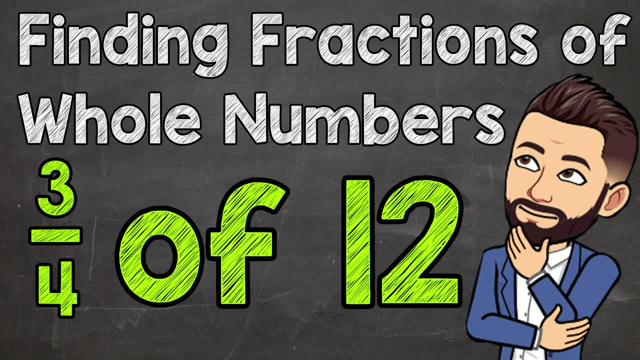 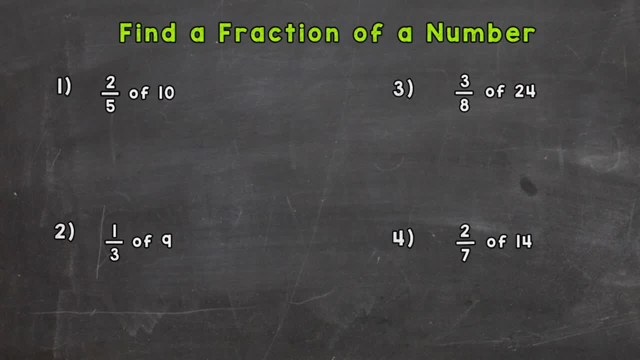 Welcome to Math with Mr J. In this video we're going to take a look at how to find a fraction of a whole number And, as you can see, there are four examples on your screen there that we're going to go through together in order to get this down. So for number one, we have two-fifths of